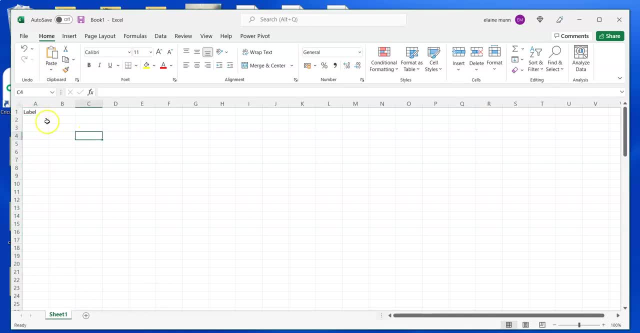 Or you can put in your number, You can put in a formula which would be put your number in there, which would be say 145.. And there you're going to put in your formula, which is equals your 145, and then your plus one. Hit your enter key, Drag it down, Okay, and it'll give you your sequence number. 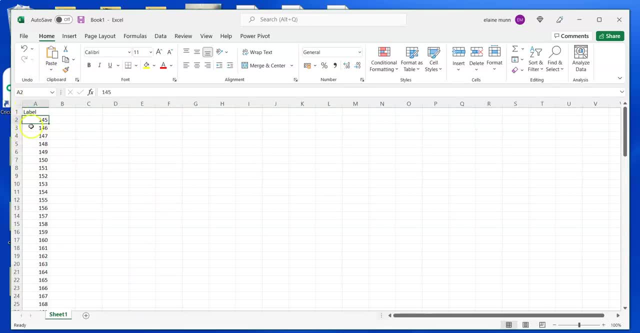 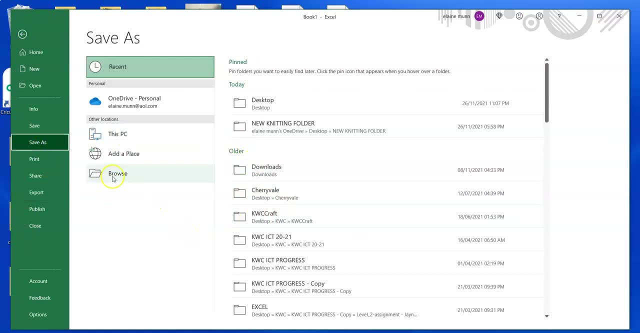 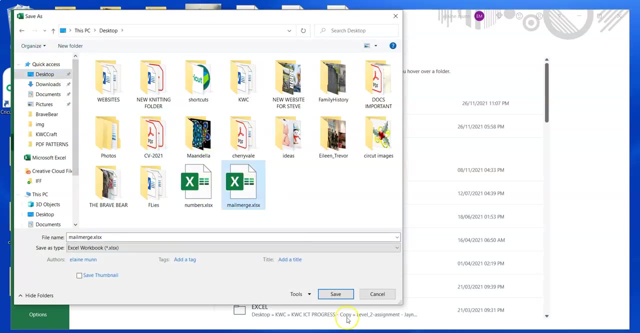 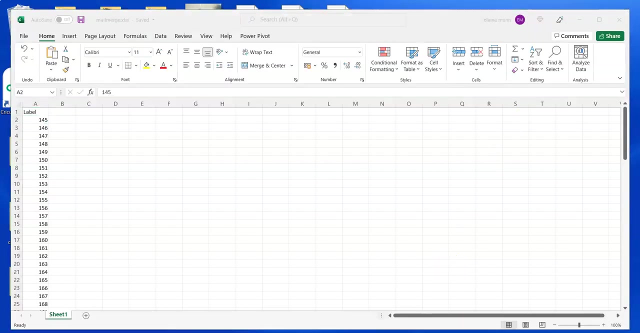 Okay. so once you've done that, you're going to put in your number. Once you've done that, once you've decided what way you want to put your numbers in, Okay, then you're going to file and you're going to save it as I just save it as, save it on the my desktop as mail merge. Okay, but call it whatever you like. Okay, so once that's done, you're going to open your Word document, a blank Word document. 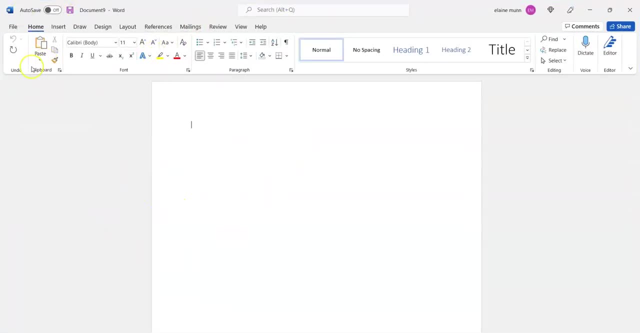 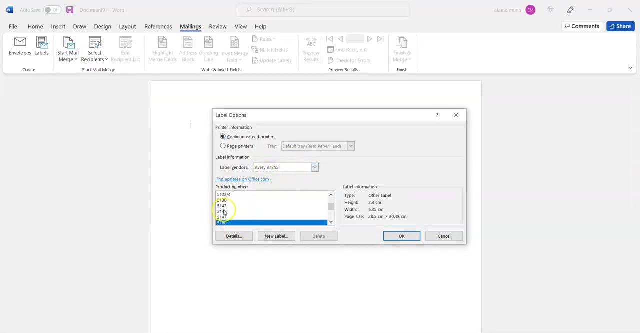 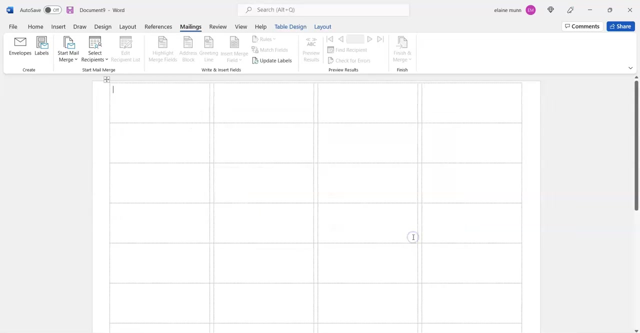 Right, and once you have your blank Word document open, you're going to go to mailings, Start mail, merge labels And that's where you'll choose the labels that you want to have. We're just going to keep it on that, but you'll have a number to choose and you go: okay, Right, you can view the grid lines. 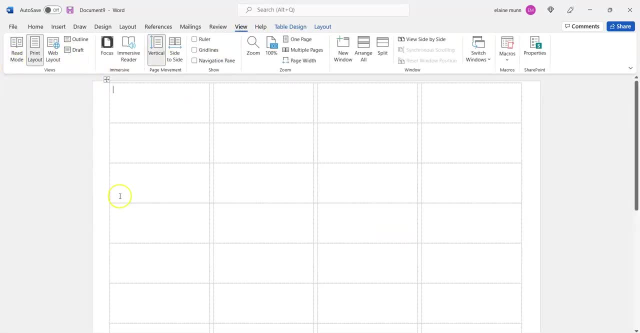 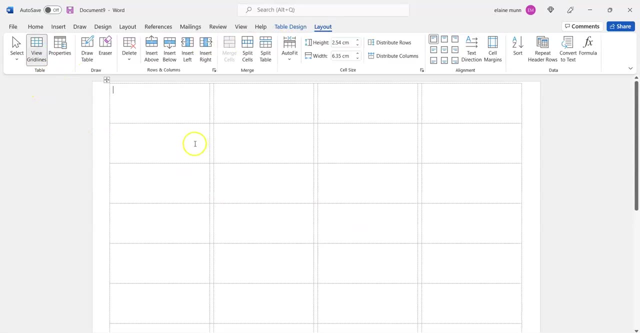 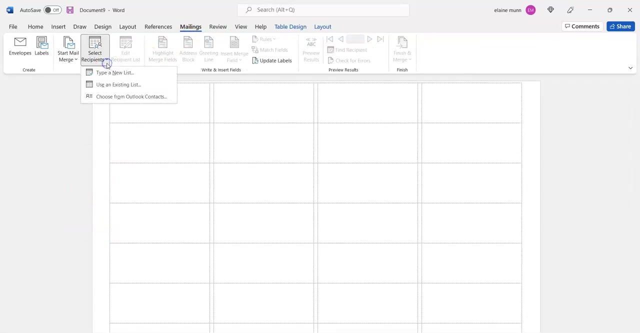 All you can actually hit save, get rid of your grid lines. so it's in. now it's in layout view grid lines. put them on. I think they're handy on. but you go back to mailings at this stage and you go to select recipients. use an existing list. I'm going to go to my 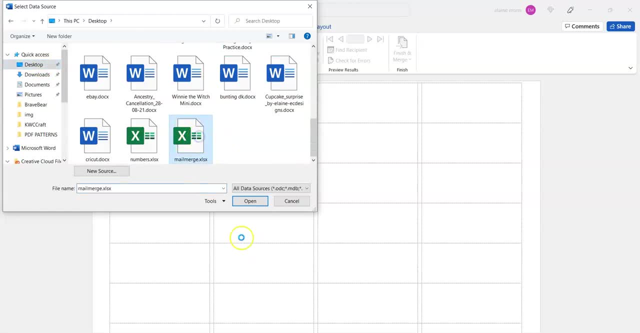 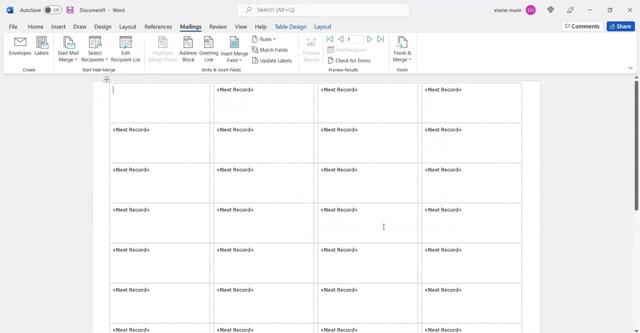 desktop where I had my saved my mail merge and open. okay, and I'm going to go: okay, puts it in there, all right, but in here you need to put in insert merge field, okay, and I want to put in label, and when you get this label up, this is: